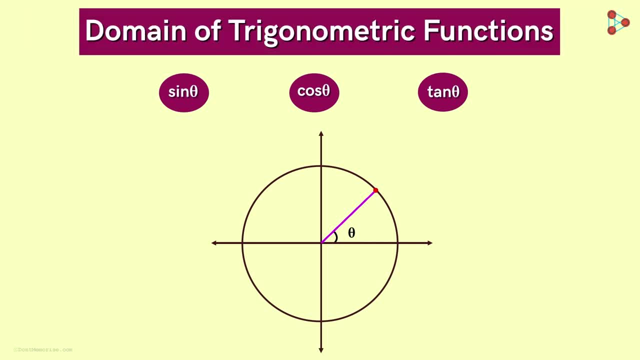 We are going to begin by understanding the domain of these functions first. We are looking for all the values of theta that can go in as input for these functions. Let's begin by finding the domain for sine theta and cos theta. Now, sine theta can be written as sine theta over 1. 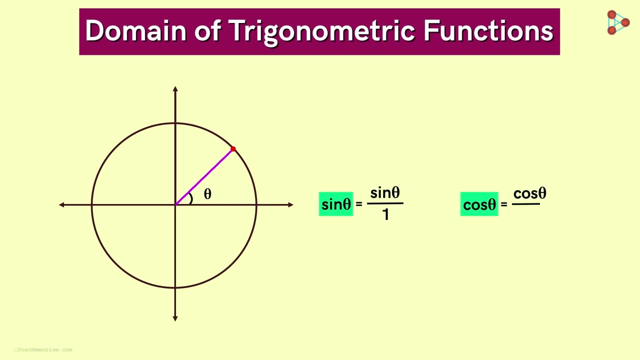 and cos theta can be written as cos theta over 1.. Why are we expressing these functions like this? That's because we want to know if theta is appearing in the denominator or not. If theta appears in the denominator, we would have to exclude all values of theta. that makes the denominator zero. 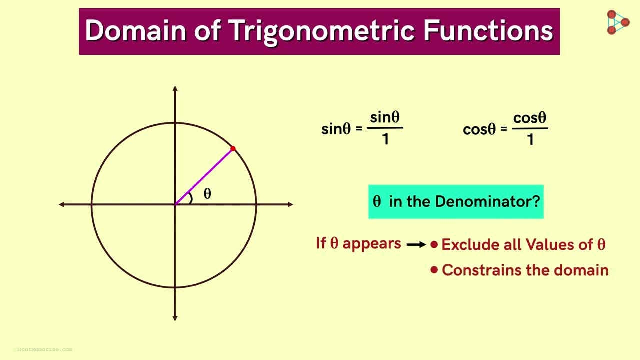 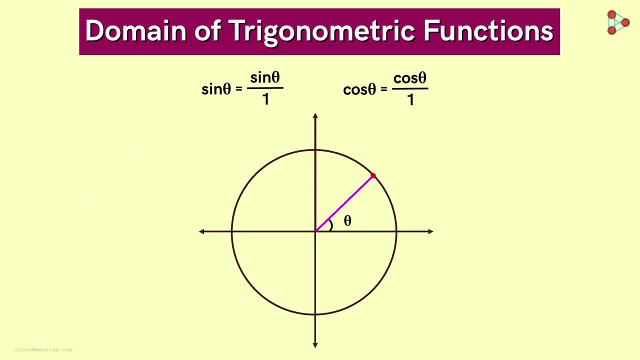 Or we can say that theta in the denominator would constrain the domain. There is no theta appearing in the denominator here. Now let's understand the domain for sine theta and cos theta. We know that when this line makes one full rotation in the counter-clockwise direction, 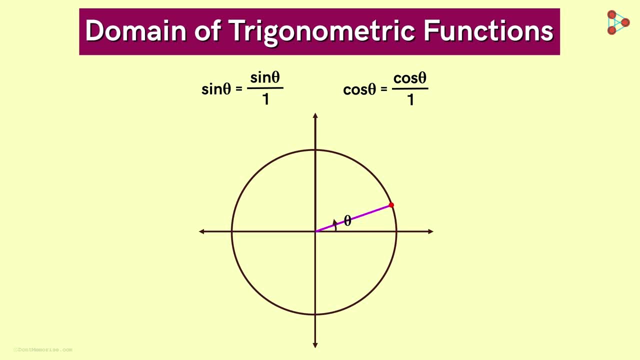 it begins at zero degrees and ends at 360 degrees. Since the rotation is counter-clockwise, the angle measurement is positive. The line can make any number of full rotations in the counter-clockwise direction, So there is no upper limit on the number of full rotations this line can make. 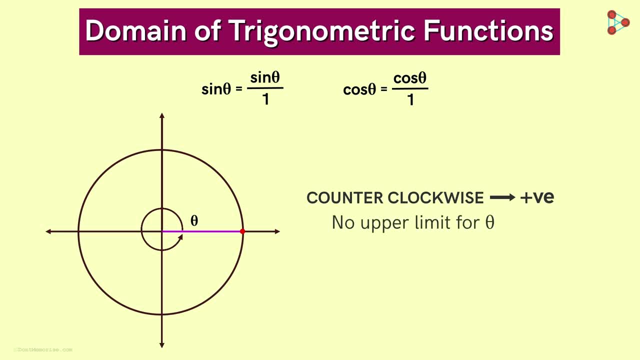 Therefore there is no upper limit for theta. Similarly, this line can even rotate in the clockwise direction, For clockwise the angle measurement is negative And similarly there is no lower limit on the number of full rotations this line can make in the clockwise direction. 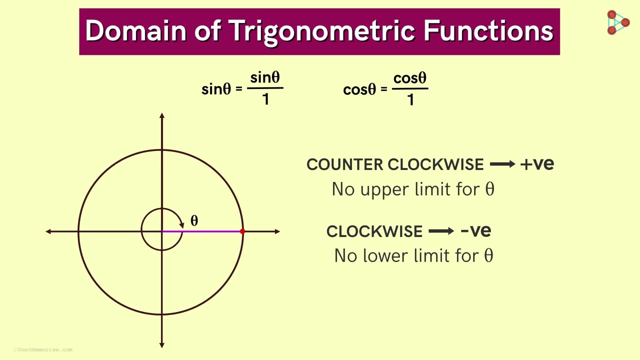 So there is no lower limit for theta. Now, mathematically, these two statements can be represented as follows: Or we can say that theta belongs to a set of real numbers, So we can say that the domain for sine theta and cos theta is all real values of theta. 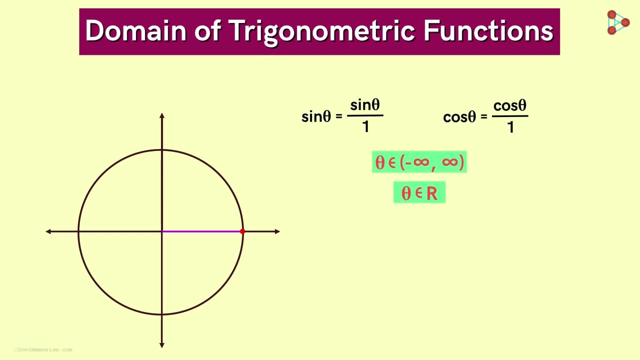 We have the domain for sine theta and cos theta. Now let's understand the domain for tan theta. Tan theta can be expressed as sine theta over cos theta. We see theta in the denominator. We want to eliminate all values of theta. that makes cos theta zero. 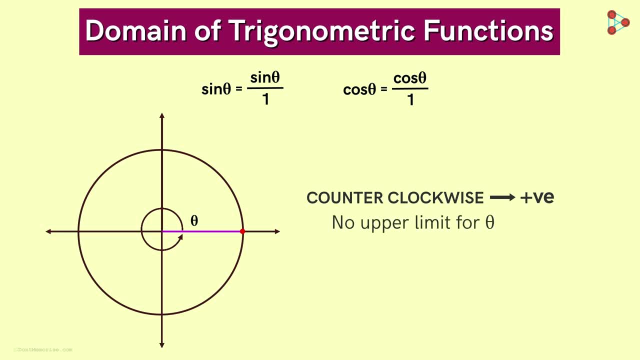 Therefore there is no upper limit for theta. Similarly, this line can even rotate in the clockwise direction, For clockwise the angle measurement is negative And similarly there is no lower limit on the number of full rotations this line can make in the clockwise direction. 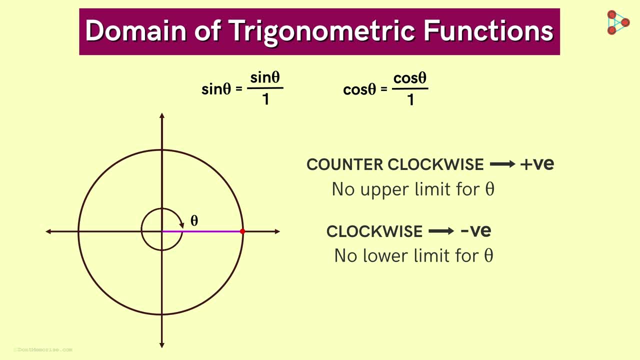 So there is no lower limit for theta. Now, mathematically, these two statements can be represented as follows: Or we can say that theta belongs to a set of real numbers, So we can say that the domain for sine theta and cos theta is all real values of theta. 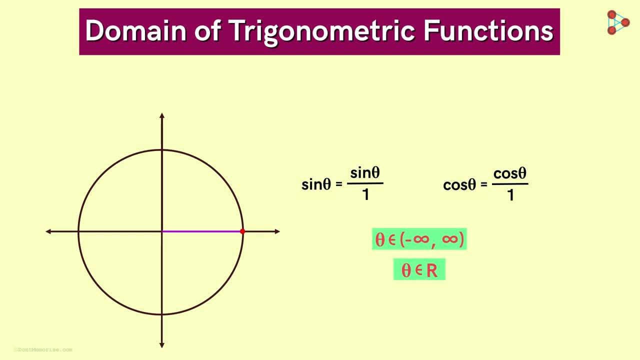 We have the domain for sine theta and cos theta. Now let's understand the domain for tan theta. Tan theta can be expressed as sine theta over cos theta. We see theta in the denominator. We want to eliminate all values of theta. that makes cos theta zero. 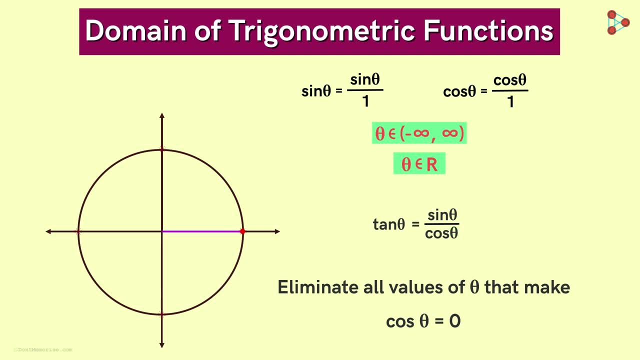 Now let's mark the coordinates of these points on our circle, On our unit circle. we see that cos theta is equal to zero. theta is equal to 0 at 90 degrees. It's also 0 at 270 degrees. In general, cos theta. 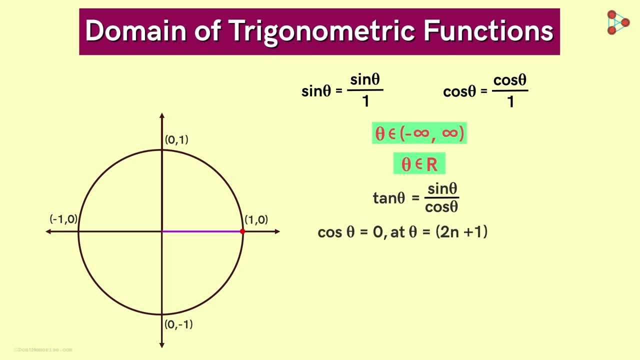 is 0 at all values of theta that are odd multiples of 90 degrees. So we eliminate all these values from our domain. Here's the domain for tan theta. In case you're using the radian measure instead of the degree measure, you can also write it like this: 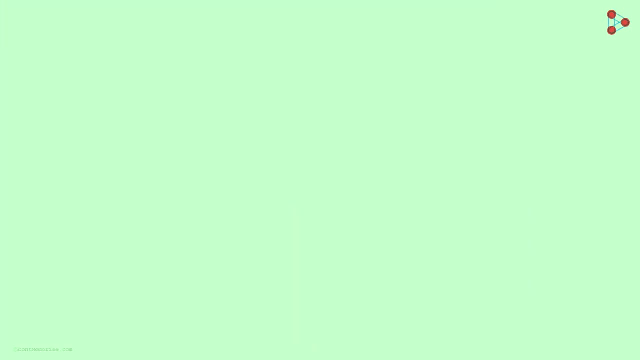 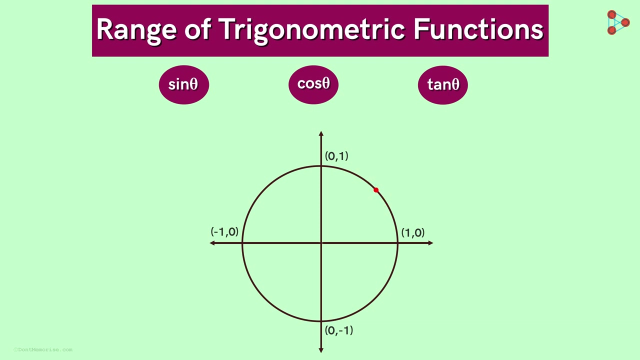 We have the domain with us. Now let's understand the range for these functions. We know that any point on the perimeter of a unit circle can be expressed as cos theta, comma sine theta. Let's look at cos theta: It's nothing but the x coordinate of this point. Now, if a point 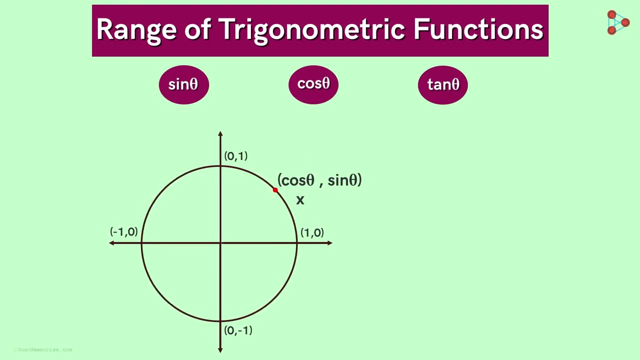 lies on the circumference of a unit circle, we can say that the maximum x value it can take is positive 1.. Now, if a point lies on the circumference of a unit circle, we can say that the maximum x value it can take is positive 1.. 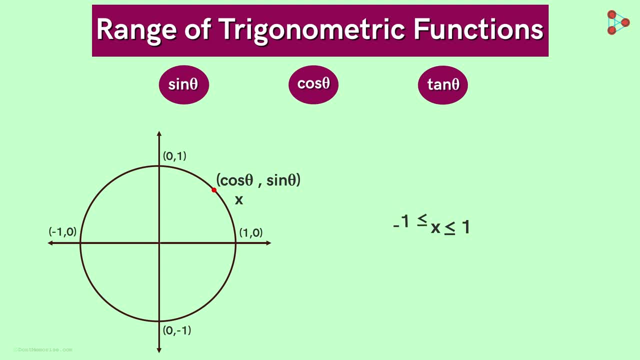 And the minimum x value it can take is negative 1.. So we can say that cos theta lies between negative 1 and 1.. This is the range of cos theta. Now we also know that the y value of any point on the unit circle is sine theta For a point. 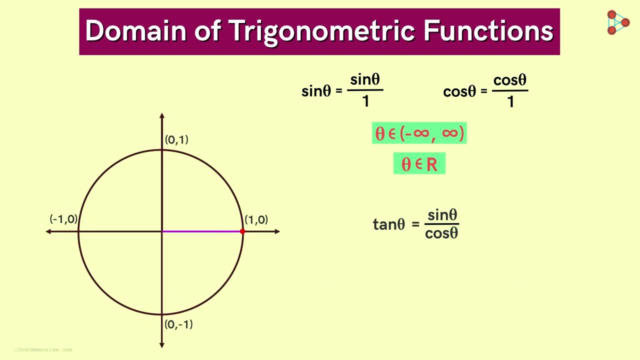 Now let's mark the coordinates of these points on our circle, On our unit circle. we see that cos theta is equal to zero at 90 degrees. It's also zero at 270 degrees. In general, cos theta is zero at all values of theta that are odd multiples of 90 degrees. 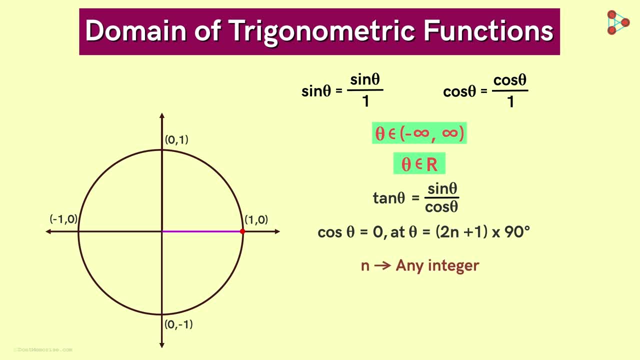 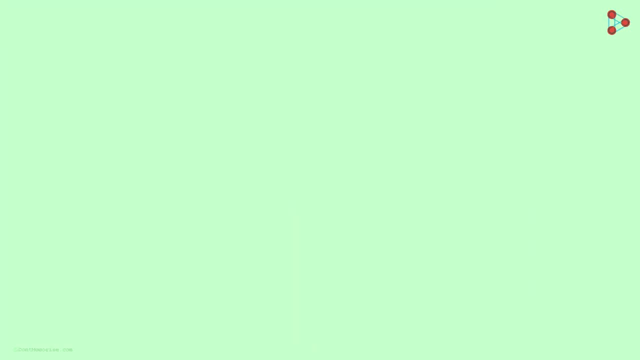 So we eliminate all these values from our domain. Here's the domain for tan theta. In case you're using the radian measure instead of the degree measure, you can also write it like this: We have the domain with us. Now let's understand the range for these functions. 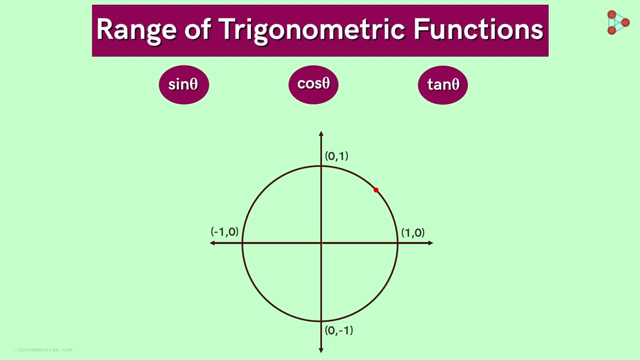 We know that any point on the perimeter of a unit circle can be expressed as cos theta, comma sine theta. Let's look at cos theta: It's nothing but the x coordinate of this point. Now, if a point lies on the circumference of a unit circle, 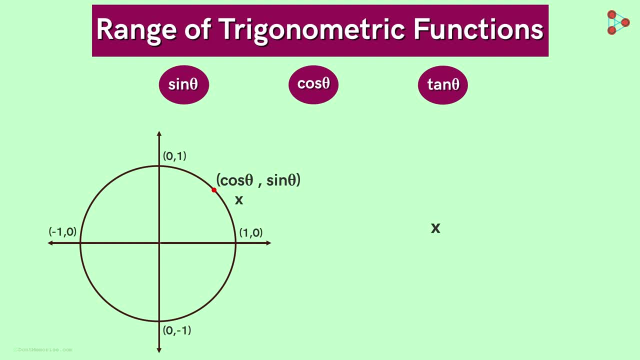 we can say that the maximum x value it can take is positive 1 and the minimum x value it can take is negative 1.. So we can say that cos theta lies between negative 1 and 1.. This is the range of cos theta. 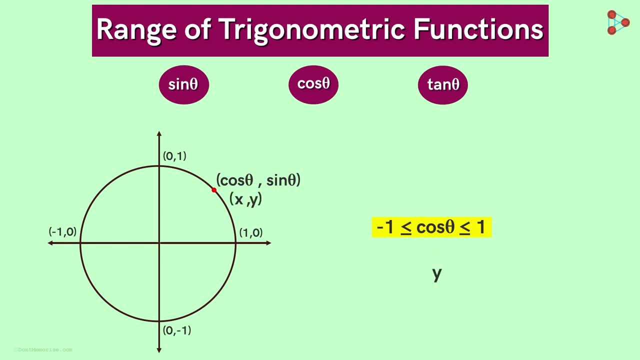 Now we also know that the y value of any point on the unit circle is sine theta. For a point lying on this circle, the maximum y value is 1 and the minimum y value is negative 1.. So the maximum y value of any point on the unit circle is negative 1.. 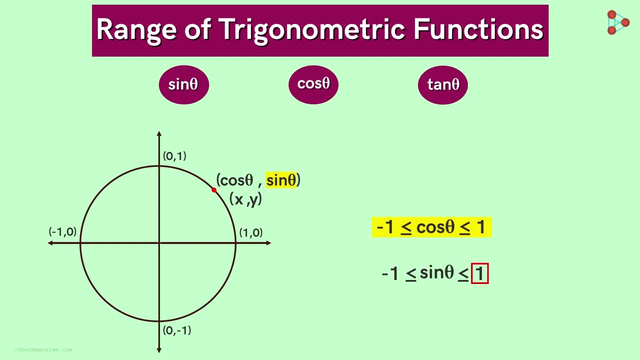 So the maximum value of sine theta is 1 and the minimum value of sine theta is negative, 1.. This is the range of sine theta. Now let's find the range of tan theta. We know that tan theta is sine theta over cos theta. 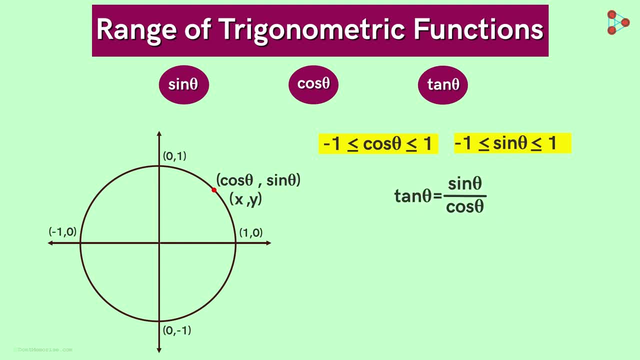 By looking at this ratio, when do you think tan theta will be maximum? Tan theta is maximum when sine theta is 1 and cos theta is 0. So tan theta is maximum here: 1 over 0 is infinity. And similarly tan theta is minimum when sine theta is negative 1 and cos theta is 0.